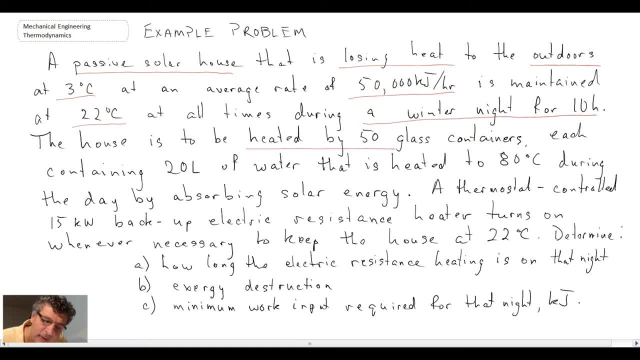 The way that we're doing this is that the house is heated by 50 glass containers, each containing 20 liters of water heated to 80 degrees C during the day by absorbing solar energy. We have a thermostat. We have a thermostat within the house that is connected to a 15 kilowatt backup electric resistance here, which turns on whenever necessary to keep the house at 22 degrees Celsius. 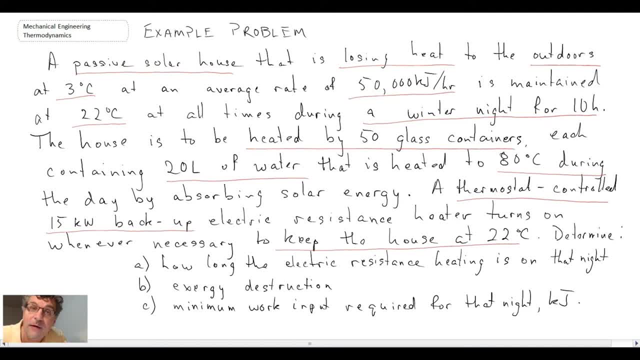 We're then asked to determine how long does that electric resistance heater need to be on during this long winter night. We're asked to evaluate the amount of exergy destroyed through this process And, finally, we're asked to determine the minimum work interval. 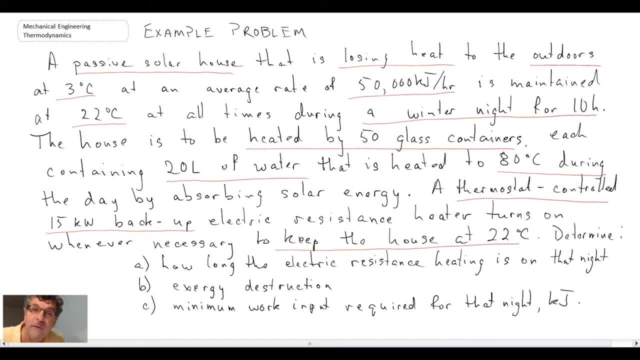 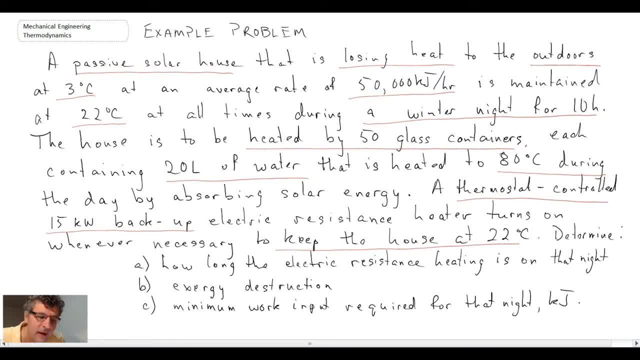 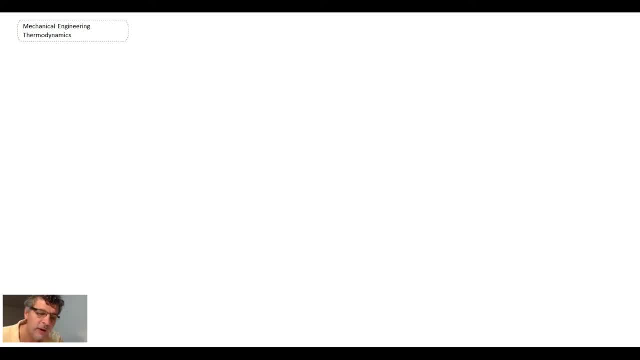 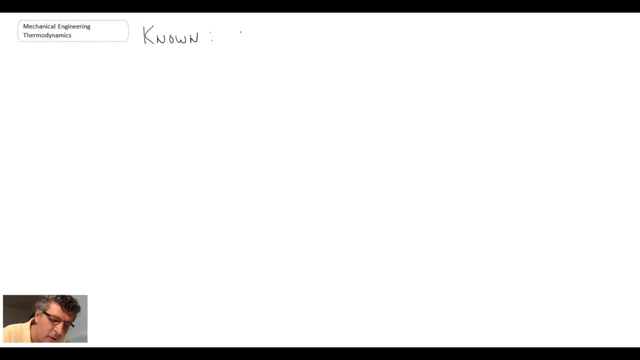 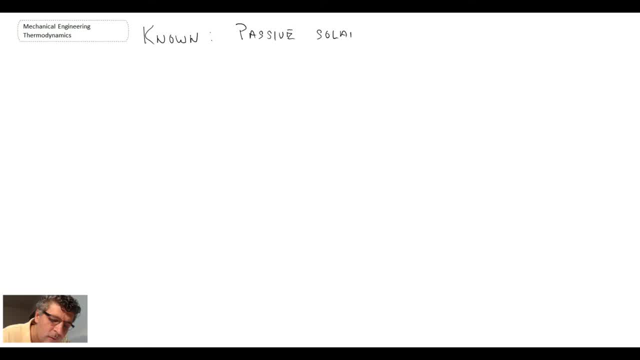 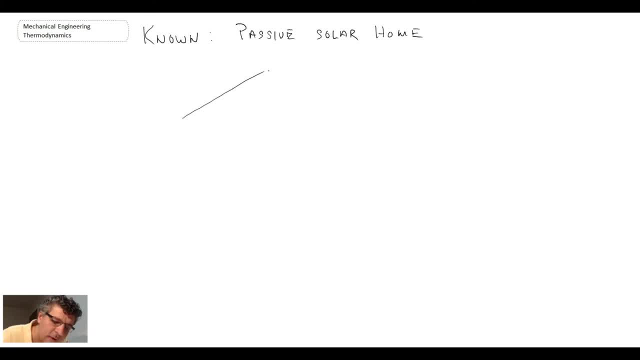 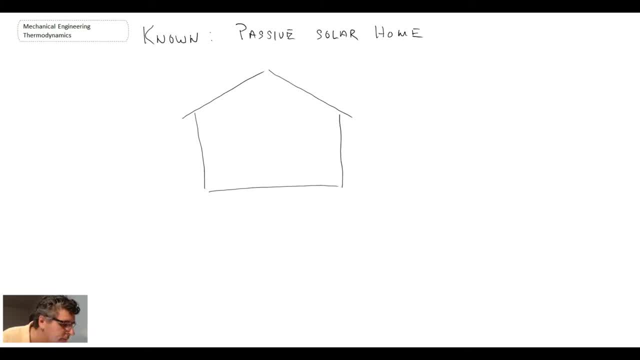 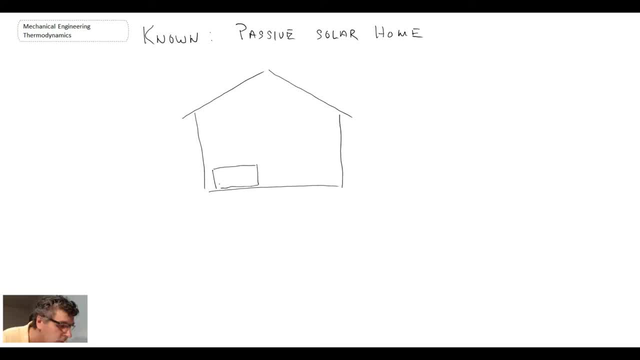 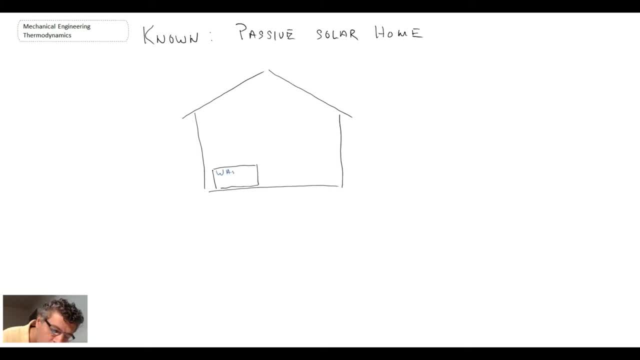 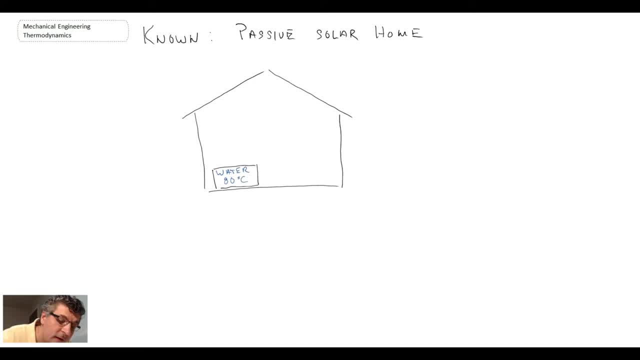 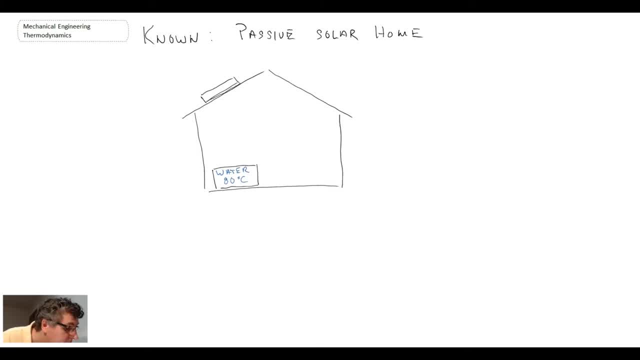 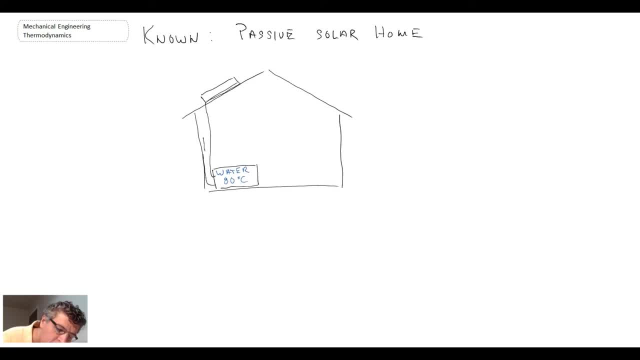 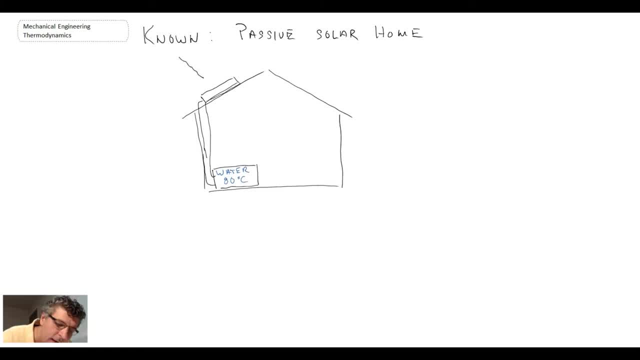 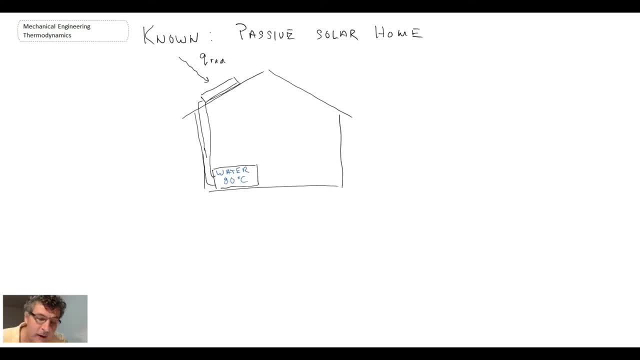 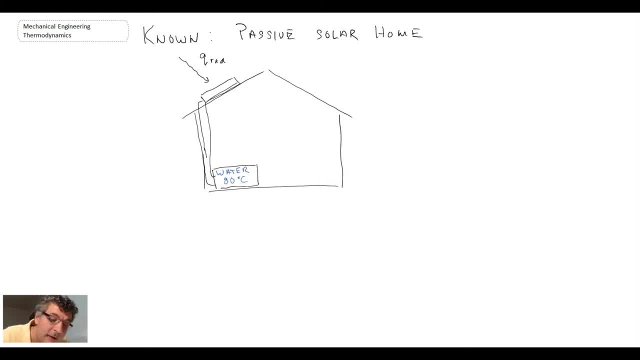 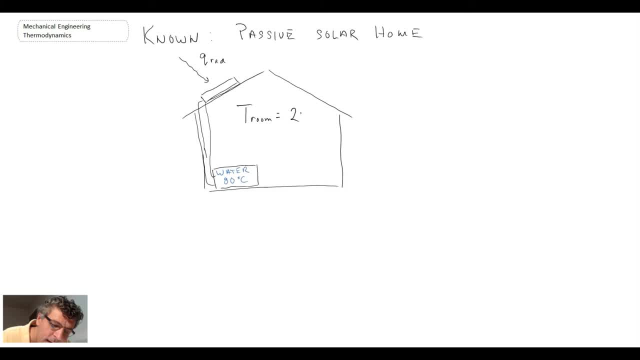 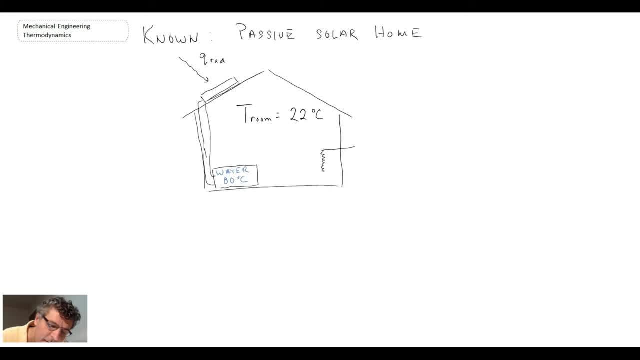 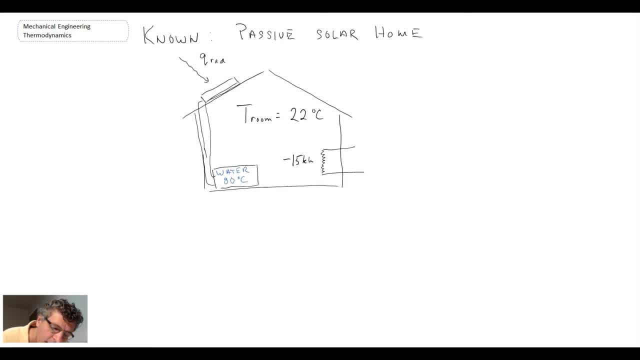 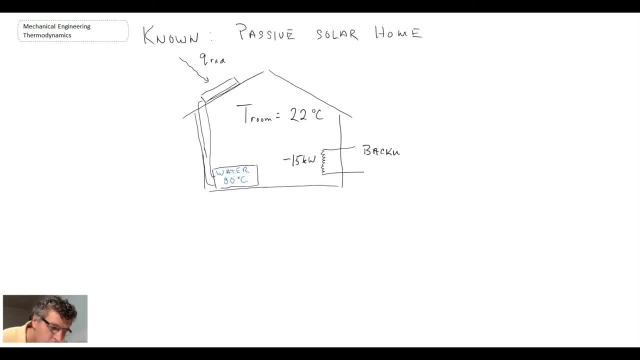 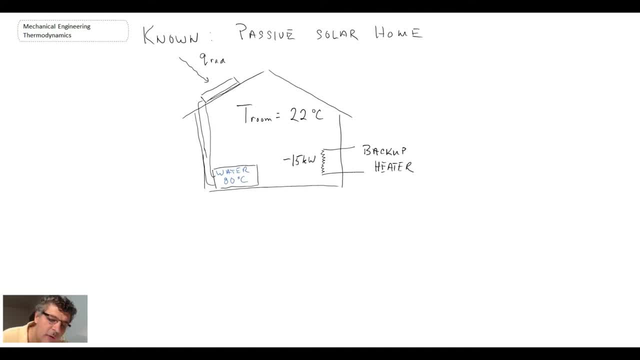 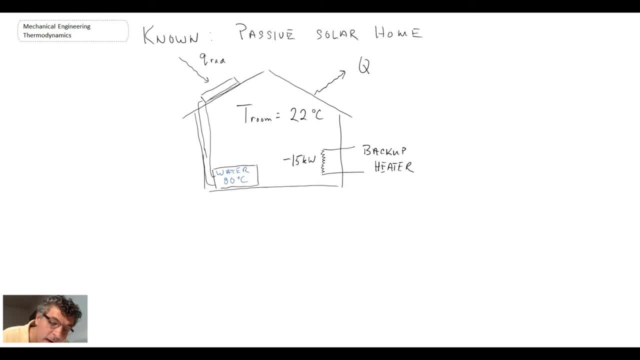 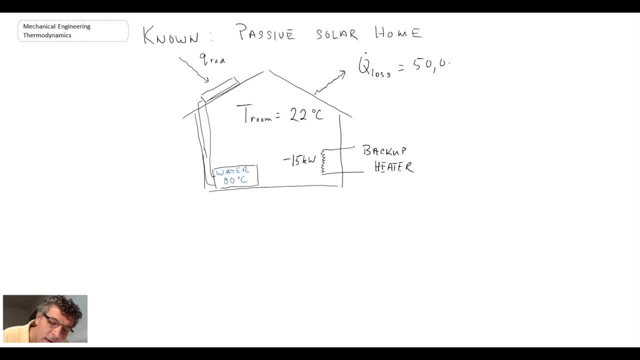 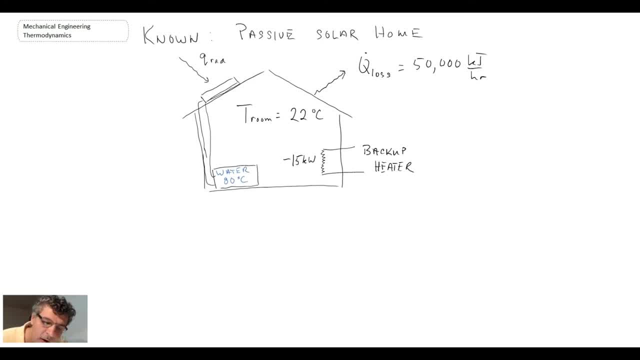 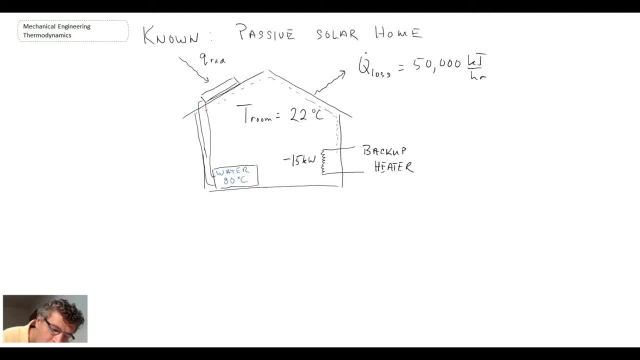 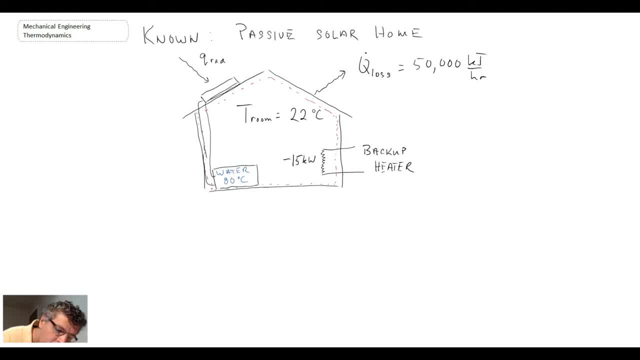 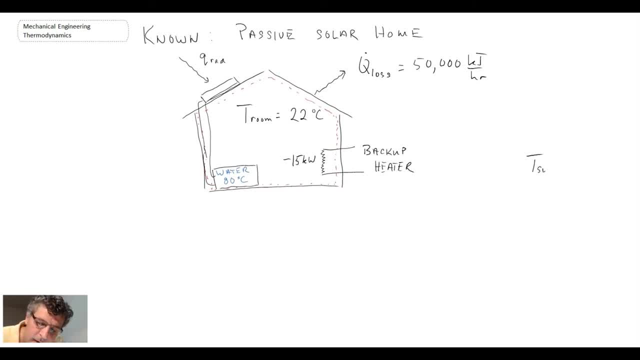 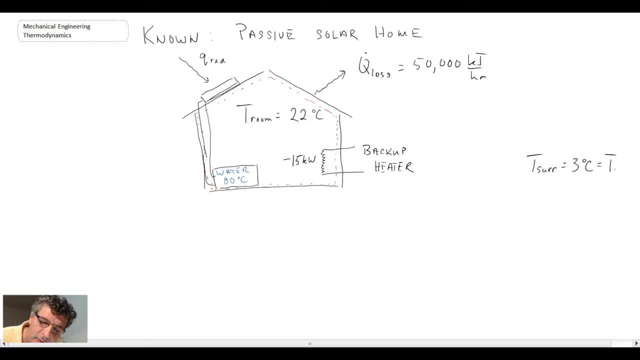 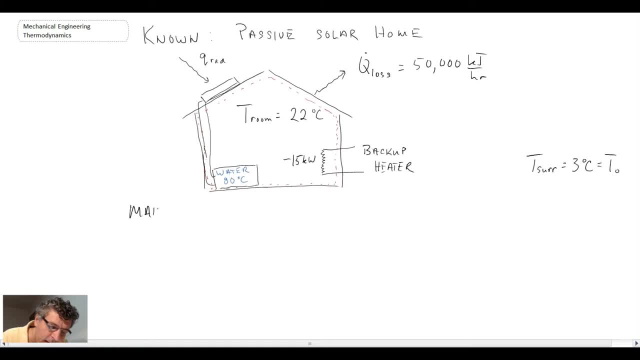 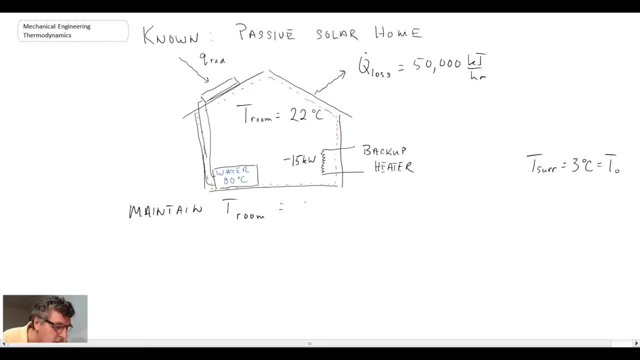 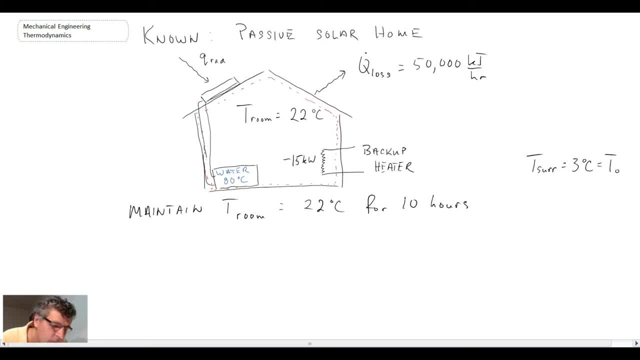 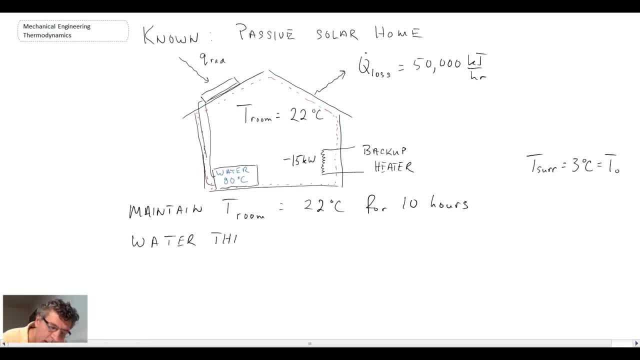 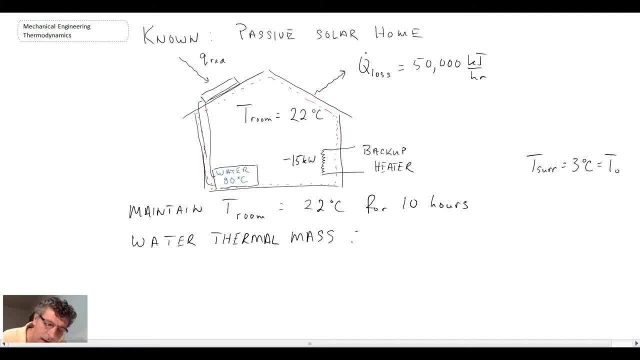 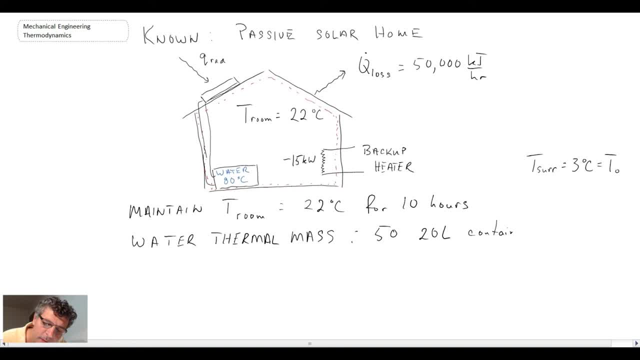 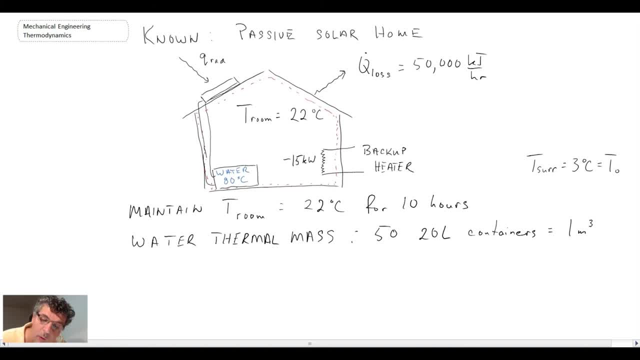 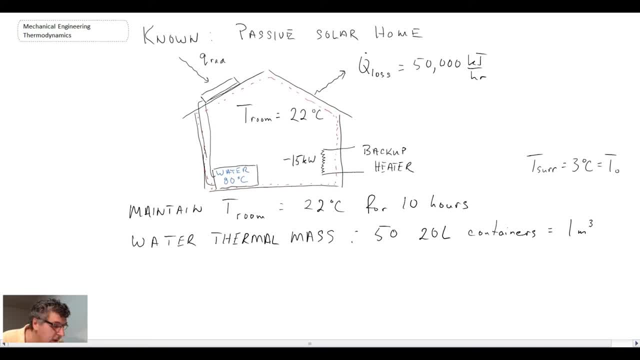 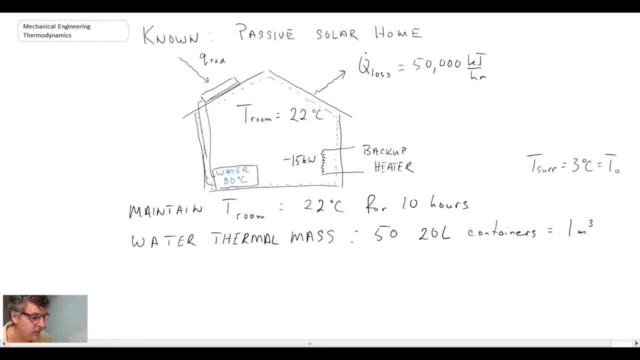 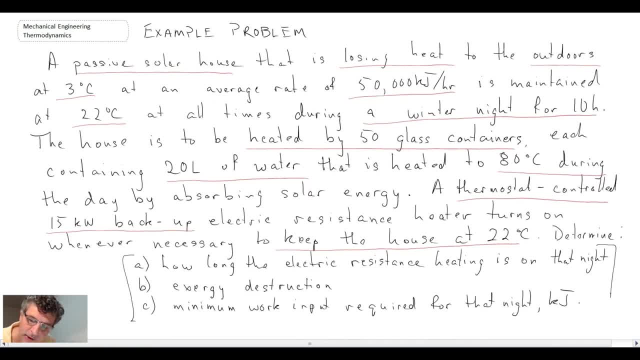 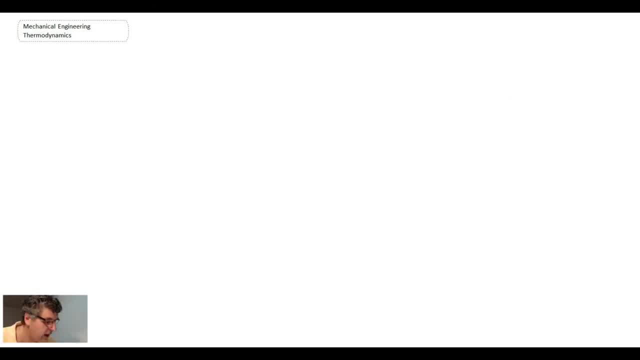 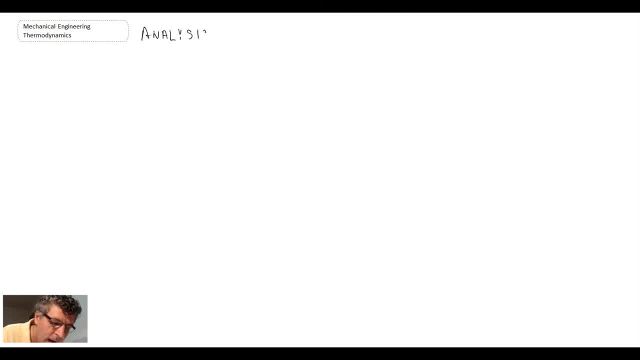 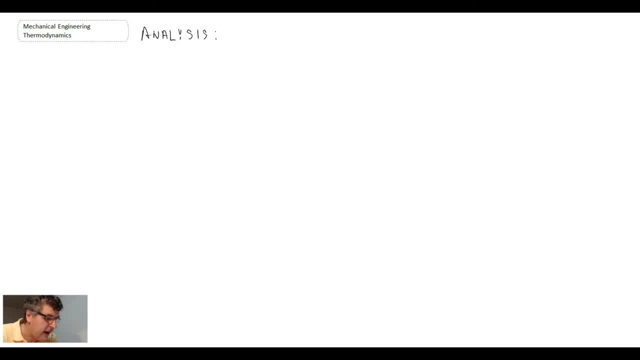 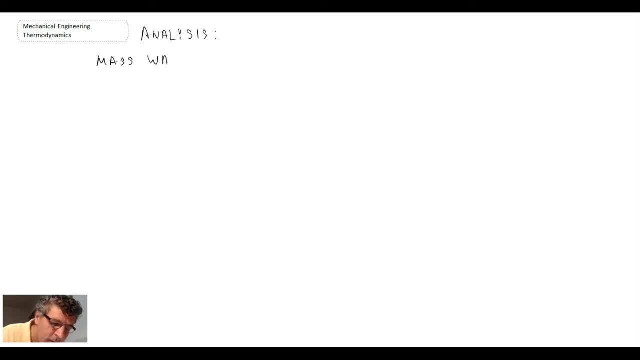 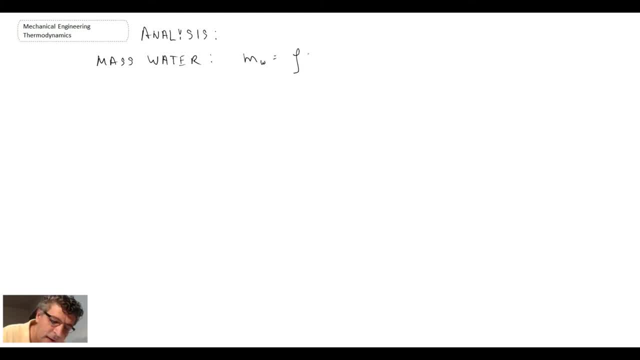 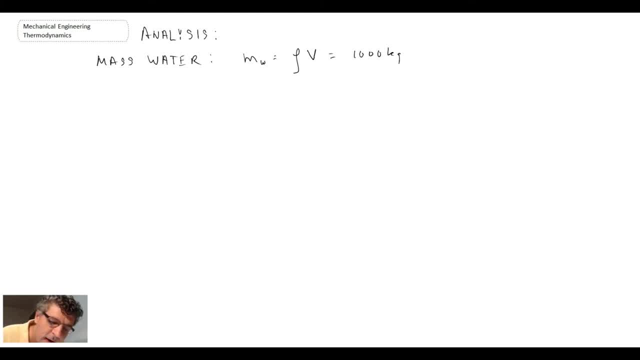 We're asked to determine the minimum work interval. We're asked to determine the minimum work interval: a thousand kilograms per meter cubed for the density of water, which is pretty close, and the volume, one meter cubed, we get a thousand kilograms for the mass of. 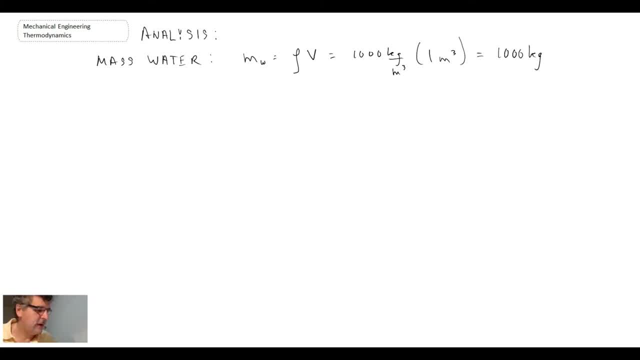 the water. so we want to figure out how long do we have to have the heating system on during the 10-hour night. we know the heat loss, we know the temperature of the water at the beginning, we know how much energy comes in through our electric resistance heater. this sounds like the first law. so 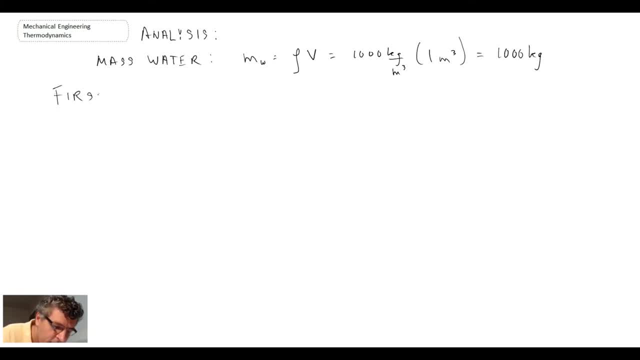 let's apply the first law, and this is going to be the first law applied to a fixed mass or closed system. okay, what can we get rid of in this equation? that's what we always do when we go through the system: these problems. can we get rid of heat loss? no, we can't. the house is losing heat. 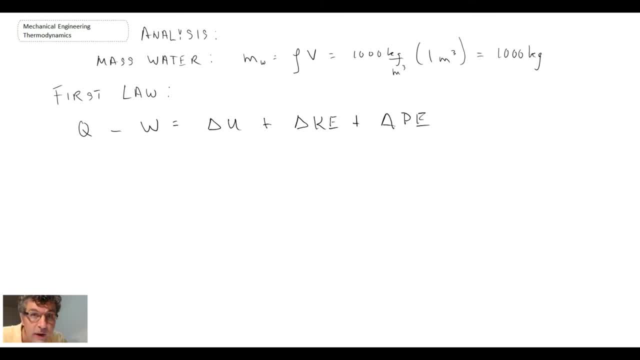 to the surroundings. can we get rid of work? no, we can't, because we have that electric resistance heater. can we get rid of the internal energy? no, we can't, because the water itself is changing temperature. can we get rid of the kinetic energy? yes, we can. the house is not moving. 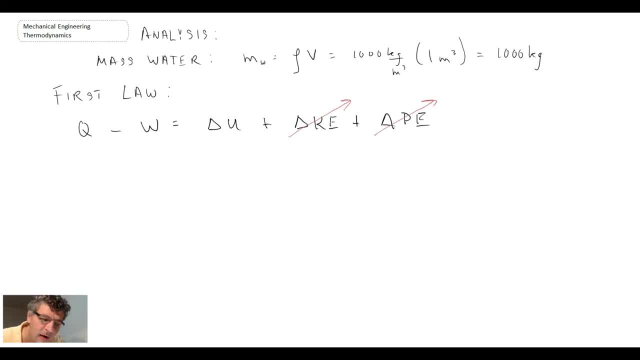 can we get rid of the potential energy? yes, again, the house is not moving. ok, so with that we whittled down the first law into something a little bit simpler, and remember the sign convention for heat transfer into a system: if the heat flows in to the system, it's positive and if the system does work, it's. 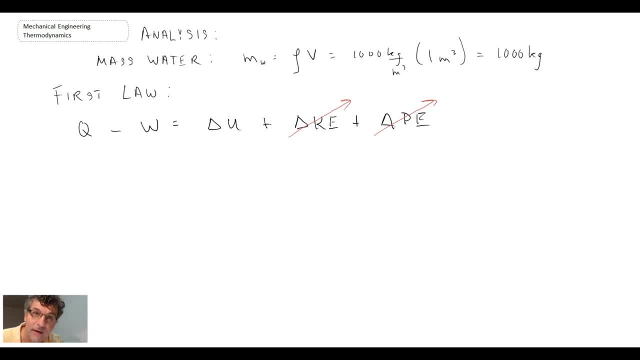 positive. in this case. we have heat leaving the system, so it's going to be negative, and we're doing work on the system, so that's going to be negative. so what we get is a minus q loss plus work. electric it's plus because it's a minus term, and then a minus w that becomes a plus. 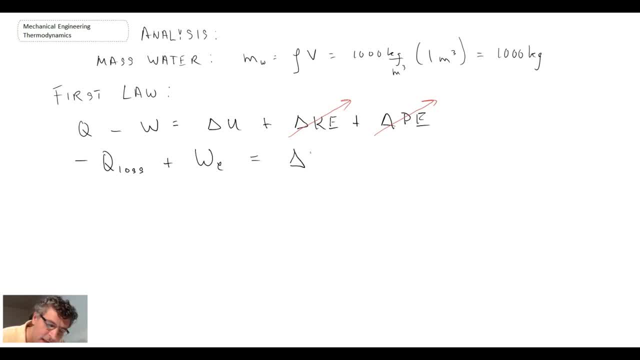 and on the right hand side we have the change in internal energy of the water plus the change in internal energy of the air, which is inside of our control volume. but wait a minute. we said the air was going to stay at 22 degrees c throughout this process, so that